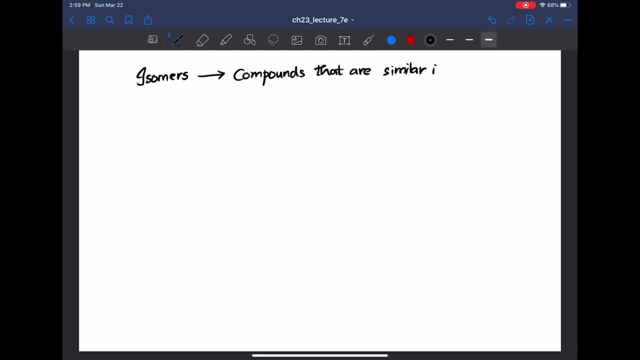 in connectivity or in optical activity. So these are called isomers in general. So there are two types of isomers, So we can classify isomers into two types. So one isomer is constitutional isomers and second is optical isomers. So let's discuss in this part 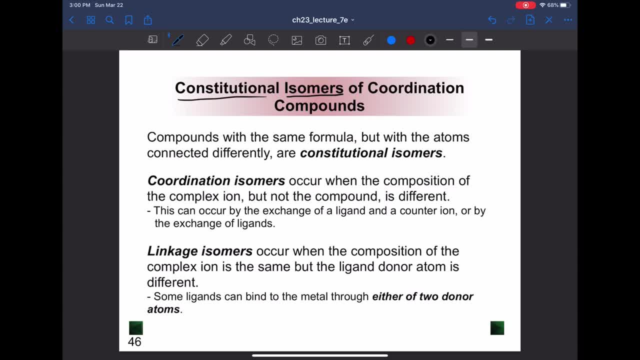 constitutional isomers first. So constitutional isomers are molecules with the same molecular formula but defer in connectivity. So here connectivity refers to the atoms ==. So these are called constitutional isomers. Now there are two types of constitutional isomers: We 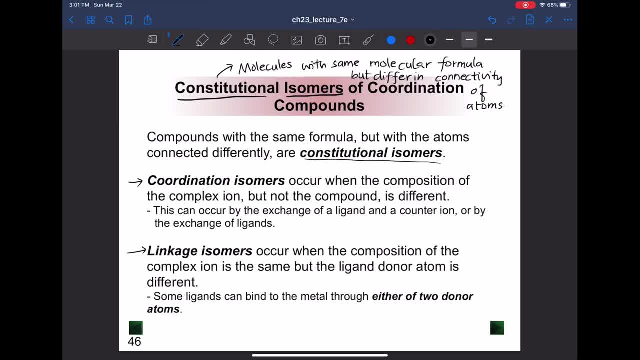 have coordination isomers and we have linkive isomers. These are we already discussed scientists isomers. Coordination isomers occur when the composition of the complex ion so occurs when the composition of the complex ion, but not the compound, is different. So this can. 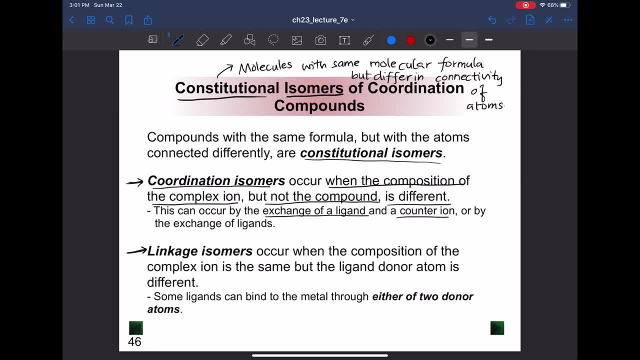 happen when there is an exchange of ligands and a counter ion, or by the exchange of ligands. So the other one is linkage isomers. so these occur when the composition of the complex ion is the same but the ligand donor atom is different. So some of these ligand atoms can band. 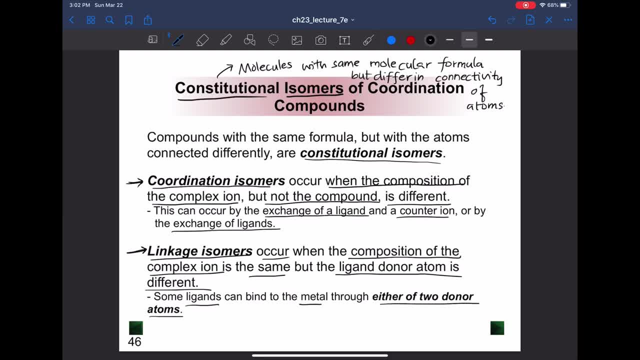 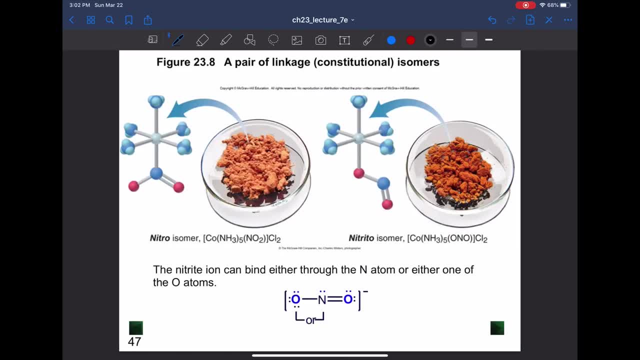 directly through the metal, through either of the two donor atoms. So the difference here is that, the difference in the linkage here, the difference in the ligand itself. Let us take an example of a linkage isomer. So in a linkage isomer you have a compound, you have this is CONH3, taken 5, NO2.. 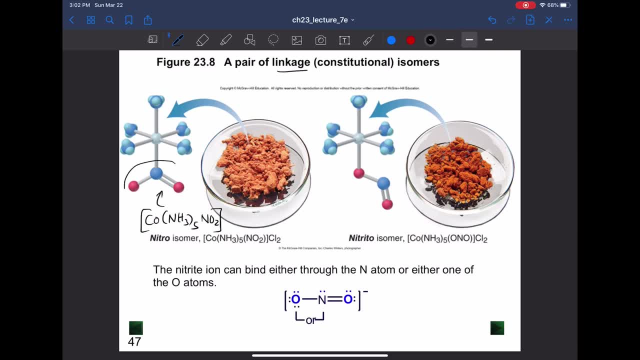 So this is the part of the complex ion, this structure. Notice that here this NO2, in this the nitrogen, is the one that is connected. Here also the internal structure is still the same. so the internal ion, the complex ion, is still the same, but here the linkage is not with nitrogen but with. 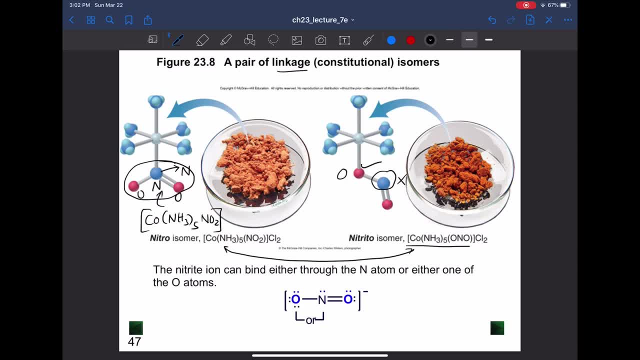 oxygen. So you have NO2. here you have ONO. So this is an example of a linkage isomer. So the one with NO2 is called as a nitro isomer. The one that bonds with oxygen is called as a nitrate isomer. 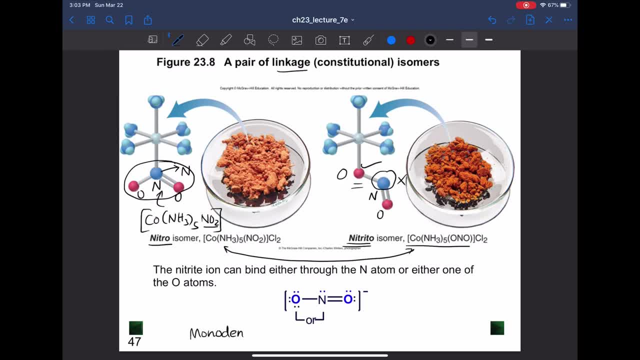 This happens in monod entendundt- weight ligands, which have more than one donor atom. so if you have two, one or more donor atoms, then this is the structure. this is the type of isomer that you will end up with with a linkage isomer. So ligands that are having more than one atom is nitrate, NaOH, nitrate, cyanide and thyosin. So ligands that are having more than one atom is nitrate, NaOH, nitrate, cyanide and thios trosonates. Let us take the number statement again. this is a linkage isomer. When they are in a linkage, this to be dimensioned here from the linkage. 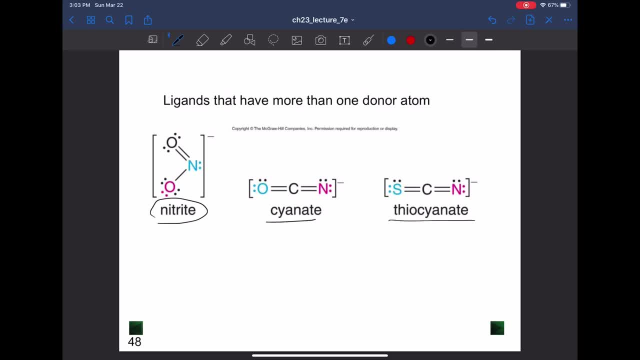 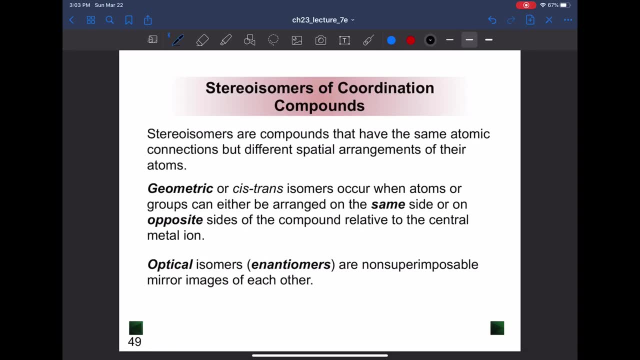 There has to be a link to an isomer, So ligands, which are't one related happening, and thiocyanate. So whenever you see cyanate, it is oxygen. Whenever you see thio, remember that it is sulfur. Next, let us look at optical isomers, So the 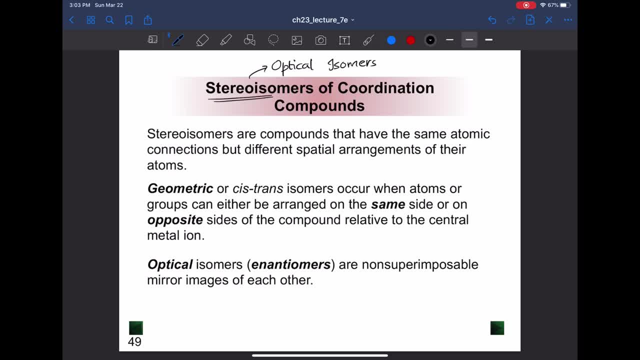 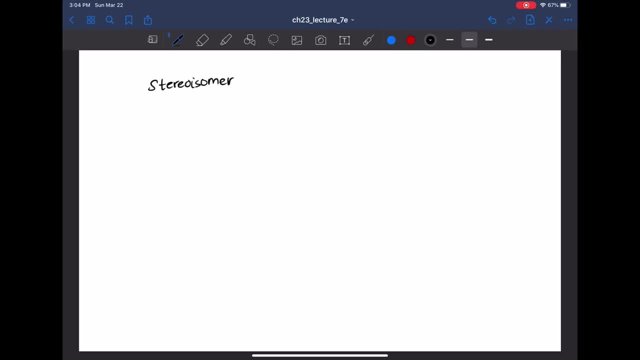 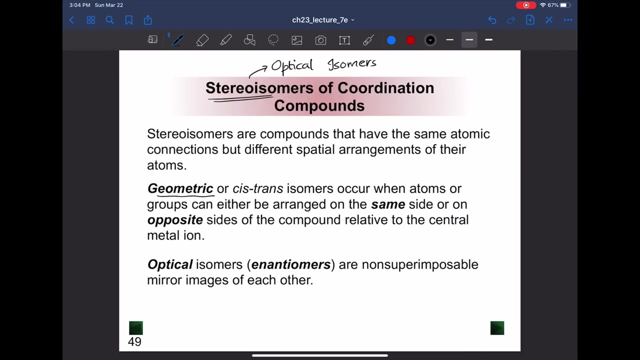 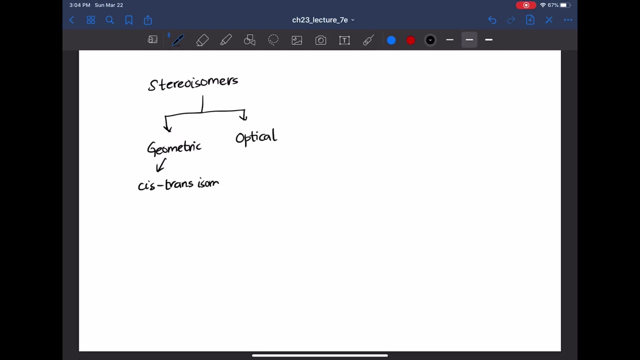 other name for optical isomers is stereoisomers. So we can classify stereoisomers into two types. One is geometric isomers, the other is optical isomers, So geometric isomers. the other name for geometric isomers is cis-trans isomers. So here, what is a stereoisomer? 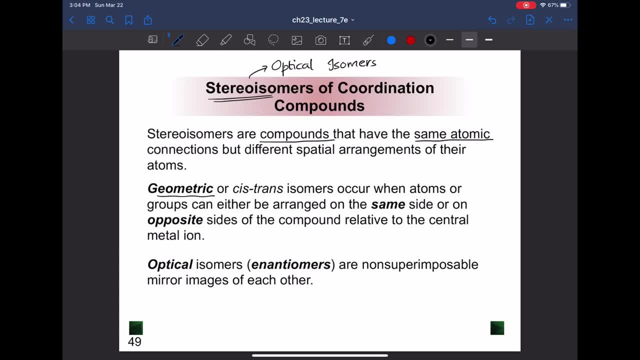 first. So stereoisomers are compounds that have the same atomic connections but different arrangements, So the one might be in the left side, one might be on the right side, So they might have different spatial arrangements. So spatial is the directions, So the directions in which 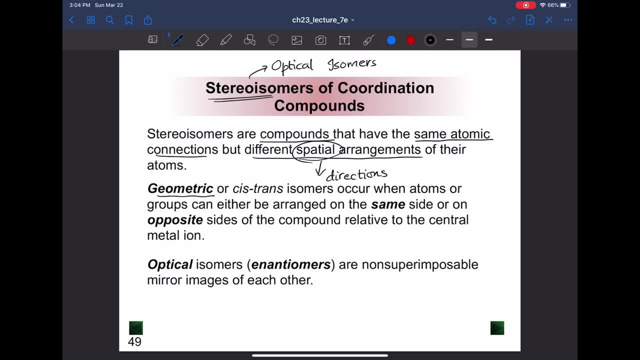 the attachments are might be different. Now, what is a geometric isomer? So geometric isomer is when the atoms or groups can be arranged on the same side or on opposite sides of the compound relative to the central metal ion. So those are called geometric isomers. 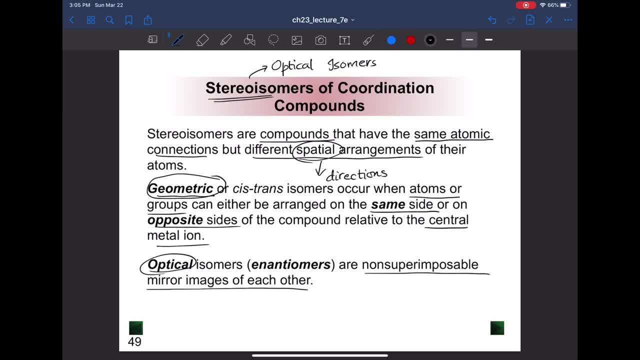 Optical isomers are basically non-superimposable mirror images. So an example of an optical isomer would be your left hand and your right hand. So if you take your left hand and right hand and put it next to each other, you notice that if both of them are mirror images of each other. but when 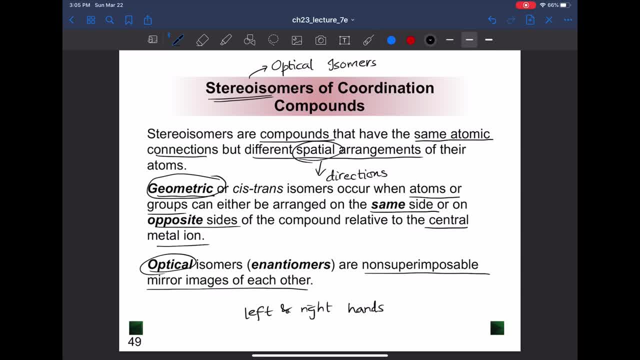 you rotate it and keep it in front of you. they are not actually similar. This is an example of a non-superimposable mirror image. So a non-superimposable mirror image is a igarebased and, as usual, a norofocal mirror image. A false one has個人 uma. 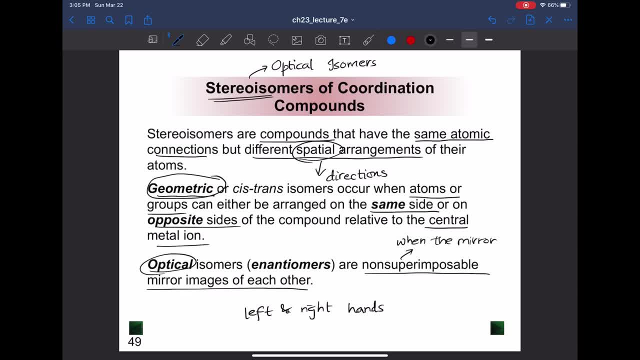 mirror image, So than instead of the mirror image we call an optical isomer. A significant pyramidod is the 티ˆisu Custom issalą. Smart mirror image is when the mirror image and the image are not the same, So mirror. 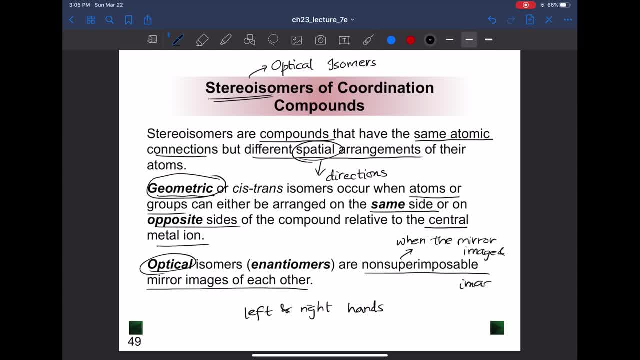 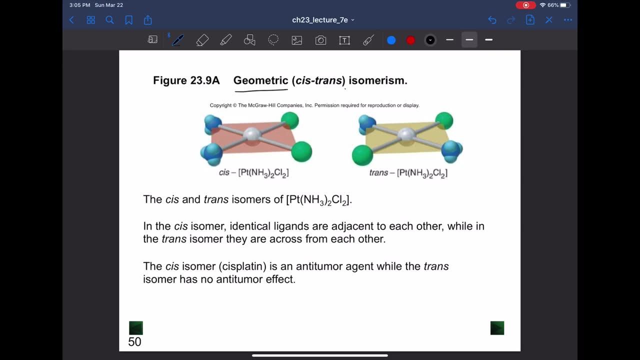 image and the image are not the same, So we call them optical isomers. Now let us take an example of a geometric isomer. So if you consider here, this is the platinum metal ion and you have two chlorines, This is where peak will go to the Atlantic place. 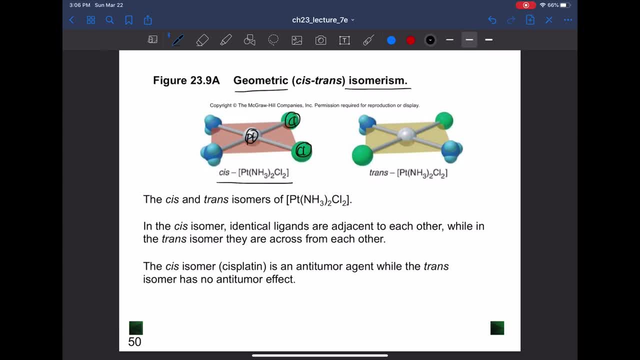 This is a metal ion in here. This is unbelievably weightless. it is報ing out the magnetic axis of the citric acid, two chlorines and you have two NH3 molecules. notice that both the groups here are on the same side. the same group are on the same side. so those are called cis isomers. if both groups 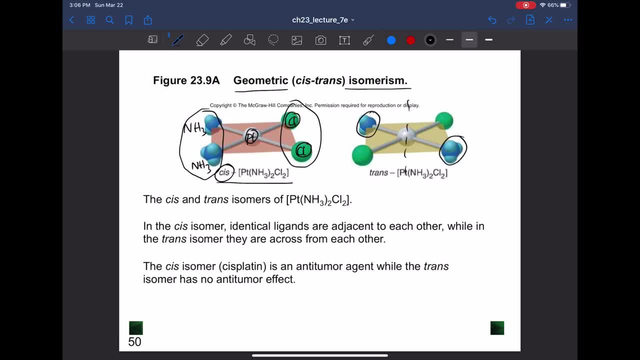 are on opposite sides of the axis of the metal ion. so to classify this, what we will do is we will cut the image in half through the metal ion and on each side we will judge whether the similar groups are on same side or on opposite side. here similar groups are on opposite. 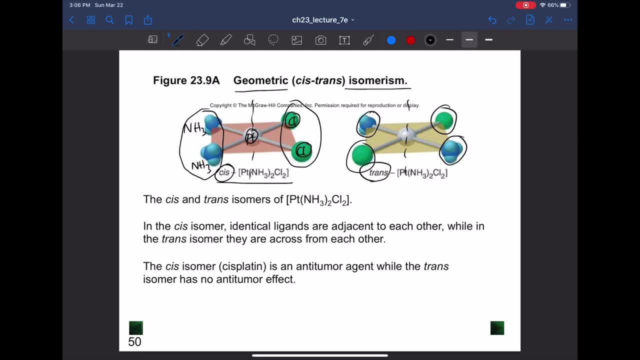 side. so we call this a trans isomer. so in a cis isomer, identical ligands are adjacent to each other. in a trans isomer they are across from each other. so best example of this would be this compound in itself. why do we need these isomers in general? because isomers in 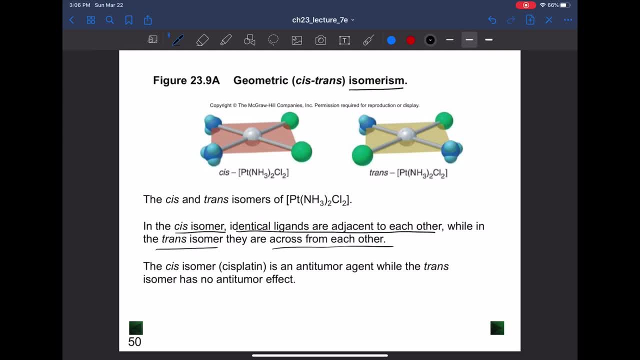 themselves can act differently in terms of the chemical reactivity. so this compound is called as a platen. The cis isomer is a trans isomer. The trans isomer of this platen is an anti-tumor agent, but the trans isomer has no anti-tumor. 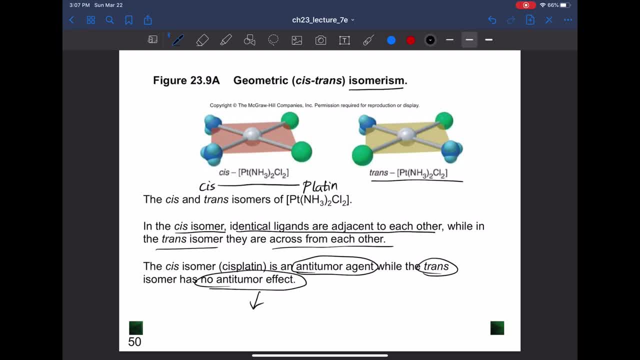 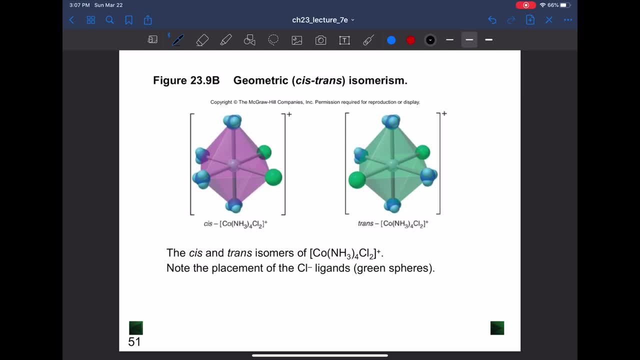 effect. so this is the reason why we have geometrical isometrism. another example of a geometrical isomer here would be to look at the axis. so if you take this compound here, you take the central metal ion. how do you classify them based on their placement is look across each. 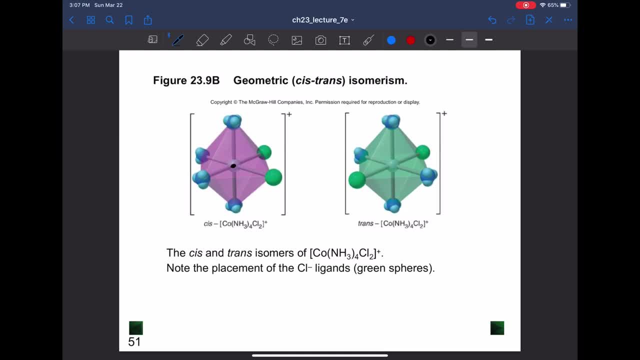 of these ions and see if, If you take in each bond, if one of them dominates where they are on the opposite sides. so if you see the linkages across the metal ion, notice that in two of them they are on the identical molecules, but then the other two, you have identical groups on each side. so 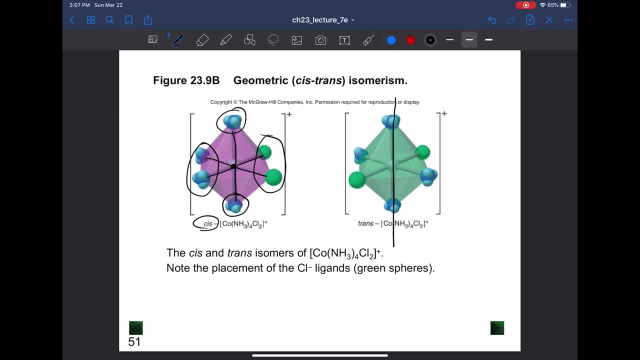 that's why it's a cis isomer. But if you take the axis here again, notice that these two are on opposite sides of each other. That is why this becomes a trans isomer. So this is how you can notate a cis isomer and a trans isomer. 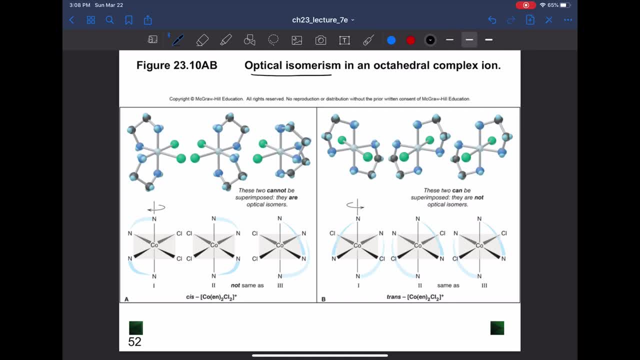 So next is optical isomerism. So optical isomerism is the mirror image concept. So if you take these two images, these two are mirror images of each other. but when you take these two, these two are not mirror images of each other. 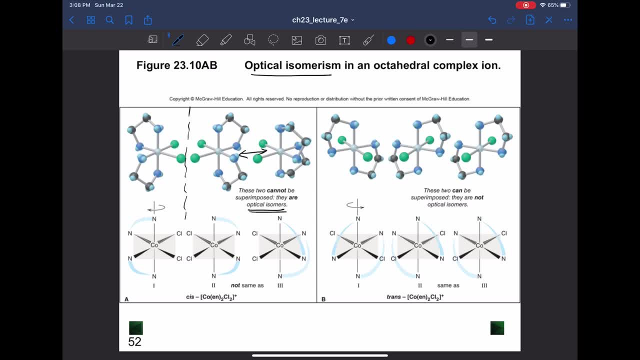 So these are called optical isomers in the same way, If you take these two, these two are mirror images of each other, but the connectivity between these two is is not the same, So they are not optical isomers, So they are only optical isomers. 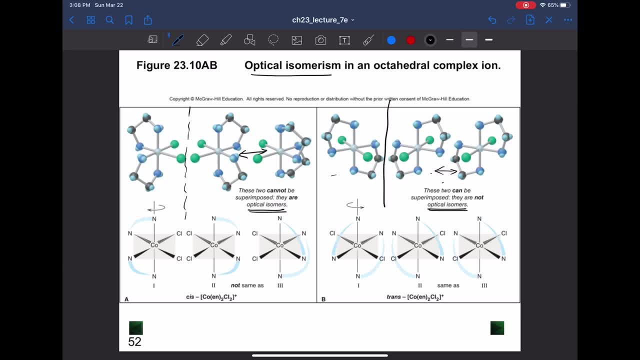 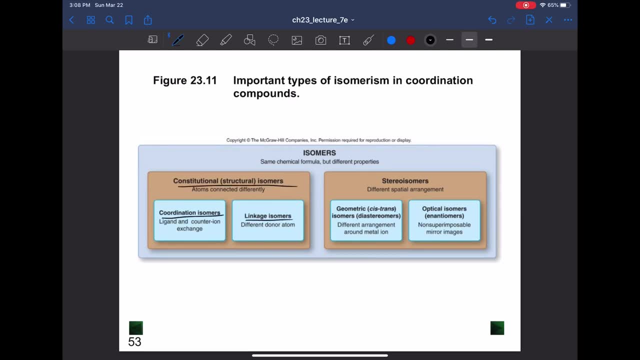 when they cannot be non-superimposable. So we can classify constitutional isomers as coordination isomers and linkage isomers, stereoisomers as geometric isomers and optical isomers, So geometrical isomers. the other name for geometrical isomers is diacetomers. 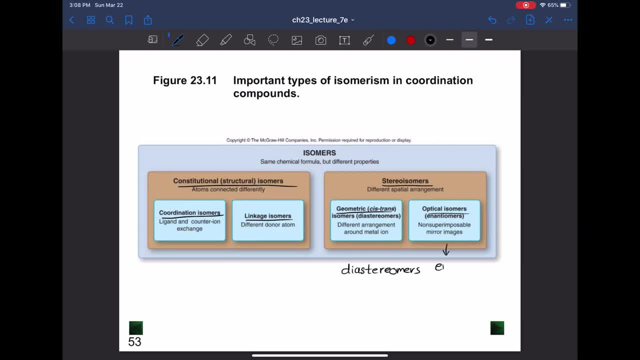 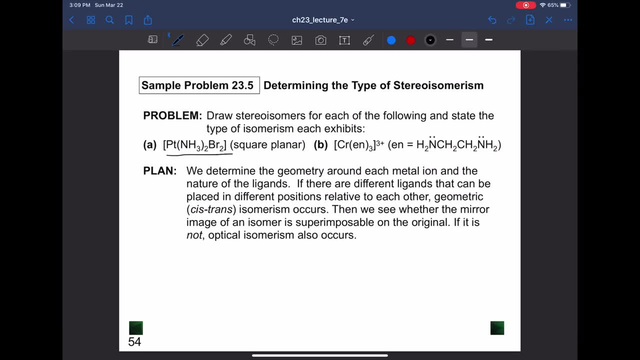 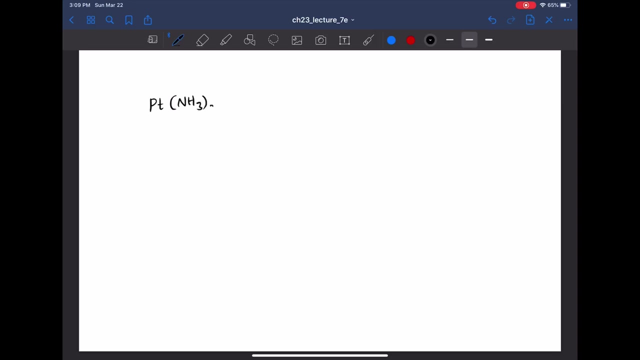 The other name for optical isomers is enantiomers. Now, try this structure. So I am going to do one, So you can try the second one. So let me try the first one. So here they are, asking you to write down the entire structures, every possible isomeric structure. So this: 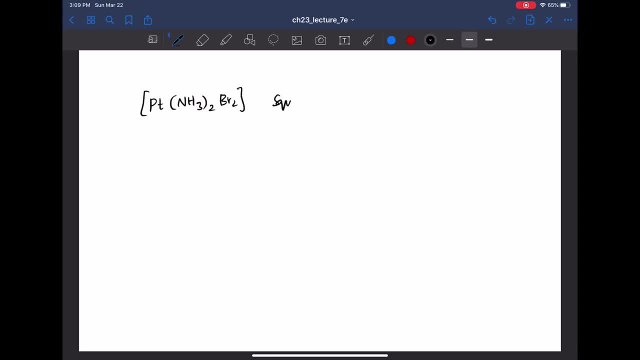 is the structure and they are giving you that. this is a Square planar structure. So in a square planar structure you have platinum in the center and you have groups on all four sides. So to differentiate this structure based on which is in the front and which is in the back, if something is on the front, we write. 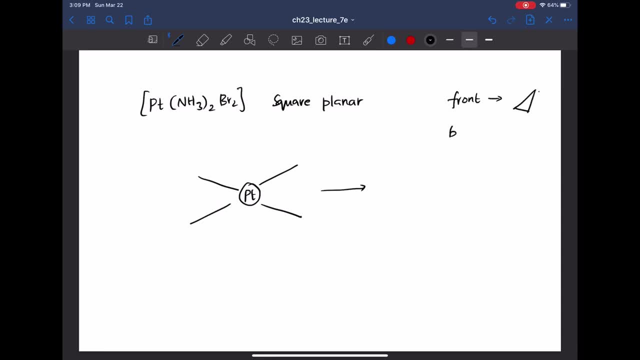 it as a wedge shape. If something is in the back, we write it as a dashed line So we can convert this structure as platinum. So we consider that the ones that are in the front are on the down and these are structures. 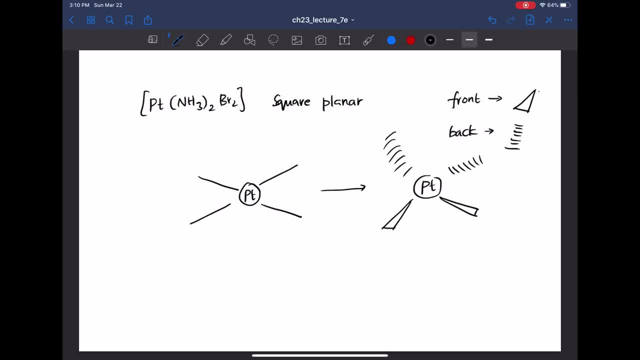 in the back side. Now we consider NH3 and Br2.. There are two chances that can happen, where NH3 can be in the front and both Br can be in the back. So this becomes cis Et. So this becomes cis Et. 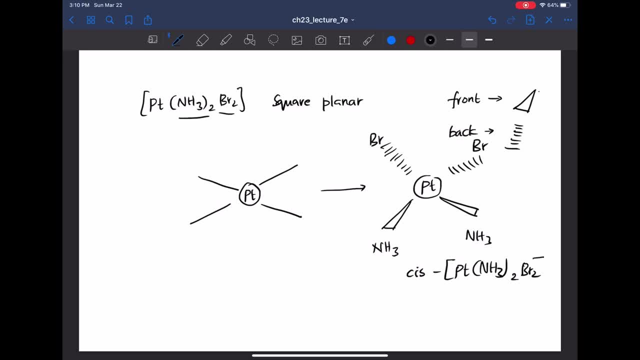 So this becomes cis Et. So NH3 taken from Br2, the trans structure for this would be where NH3 is in the front and Br is in the back. You have NH3 on this side and there is Br on this side, So notice. 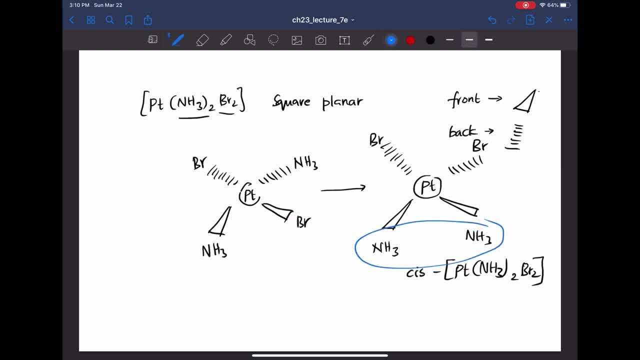 that here Both NH3s are on the same side. BR is on the back side. So this is an example of a C size number. Here NH3 and BR are on the opposite side. So that is why? So, because we are. 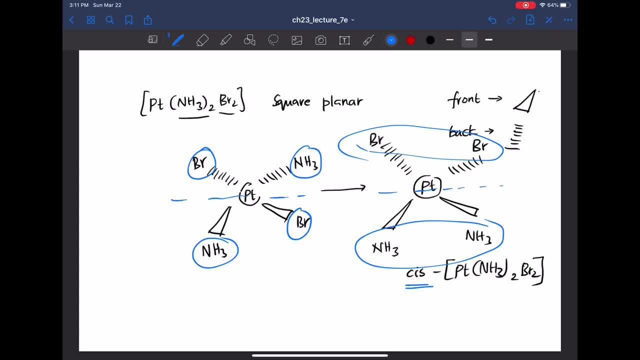 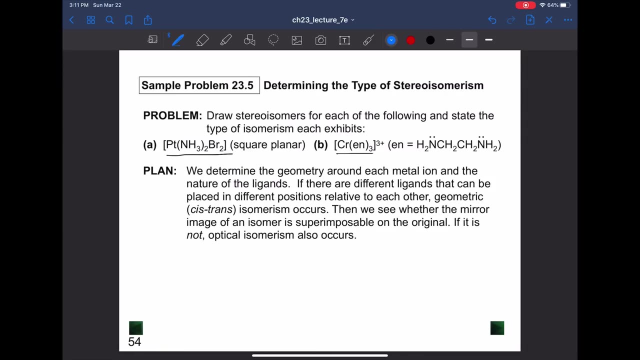 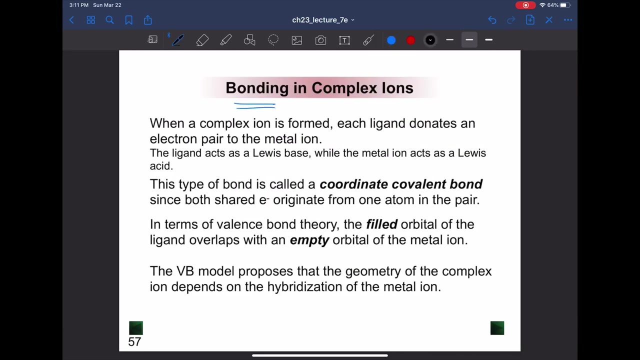 considering this axis. So this becomes a trans PT NH3, taken towards BR. So this is the structure of conditions. So what are the types of bonding in the complex ions? So when a complex ion is formed, each ligand here donates an electron pale to the metal. 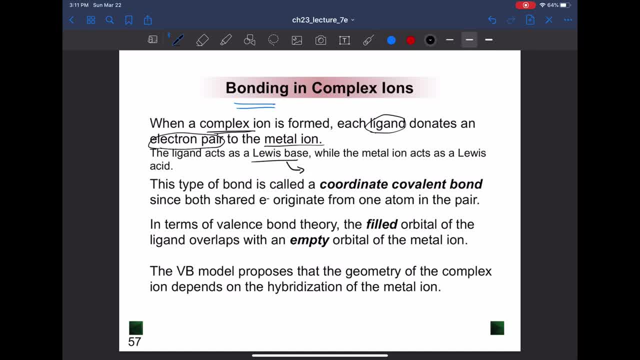 ion, The ligand acts as acts as a Lewis base, basically meaning that it acts as a electron pale donor. But the metal ion acts as a Lewis acid, meaning that this acts as an electron pair acceptor. So this type of bond is called as a coordinate. 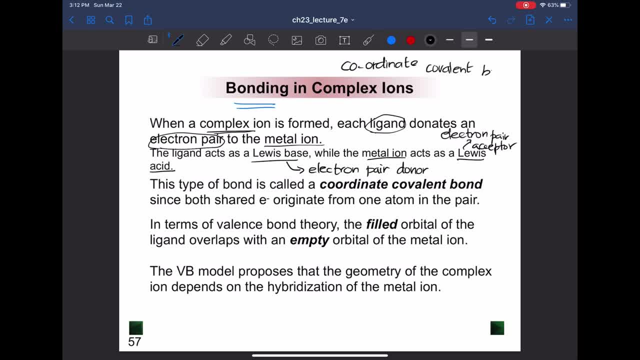 covalent bond. What is the difference between a coordinate covalent bond and a covalent bond? If you consider a covalent bond, for example, if you have carbon with four carbons? for example, let us consider that oxygen with its two lone pair of electrons. there is another. 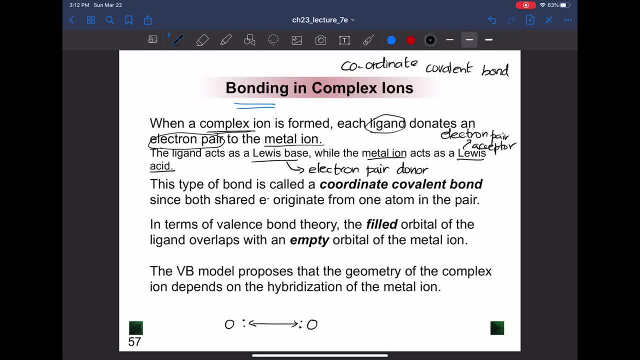 oxygen with these two lone pairs. These two like to share those electrons, So this donates its electrons and this oxygen also donates its electrons, So that results in oxygen forming double bond, In a coordinate covalent bond. only one atom donates electrons, So 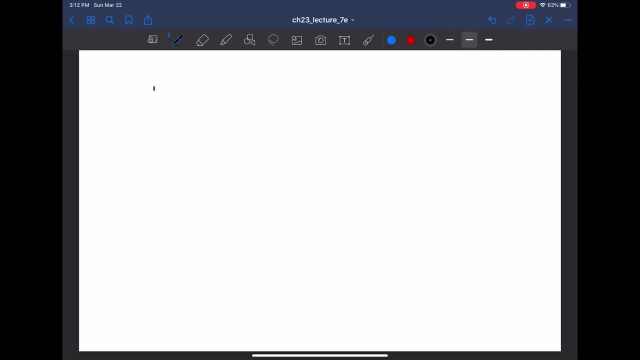 best example of this would be if you consider a structure of BH3 and NH3.. NH3 here has a lone pair of electrons, So this donates it to BH3 and then forms BH3 bond NH3.. This bond- here is a representation. 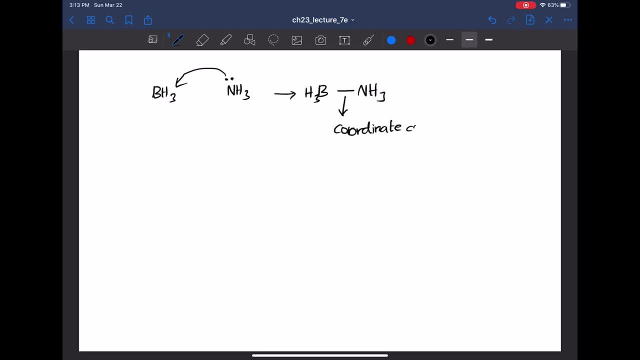 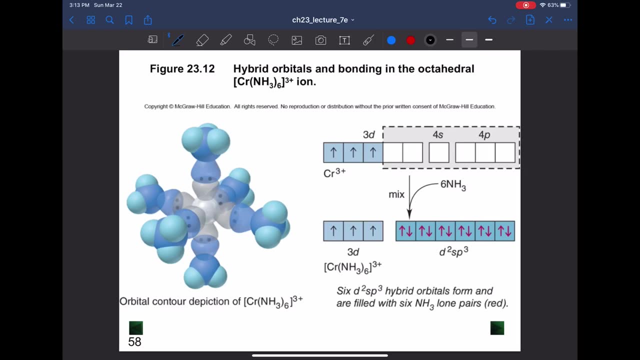 of coordinate covalent bond. So what type of hybridization would you see here? So the common hybridizations that we generally see are ASP3, ASP3D2, and you can also see ASP, ASP sometimes. So what type? 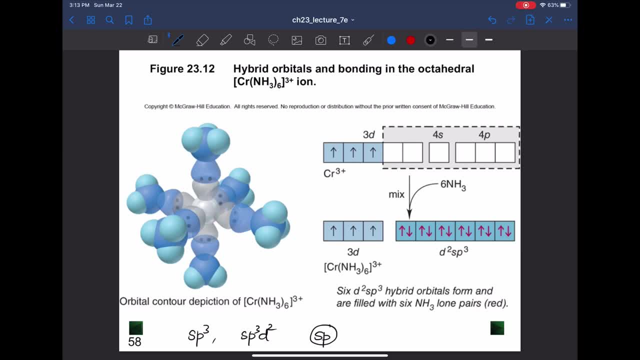 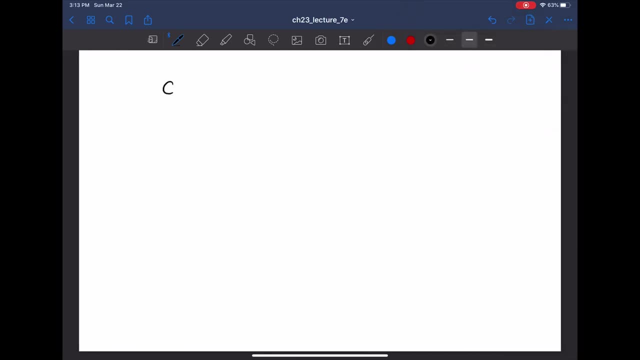 of hybridization would we generally see. So let us take an example of this atom: chromium ammoniate, so this is sorry, hexa amine chromate. So let us take this atom, CrnH3, taken 6, 3 plus, So here you have a chromium atom which is 3 plus charge, So chromium. 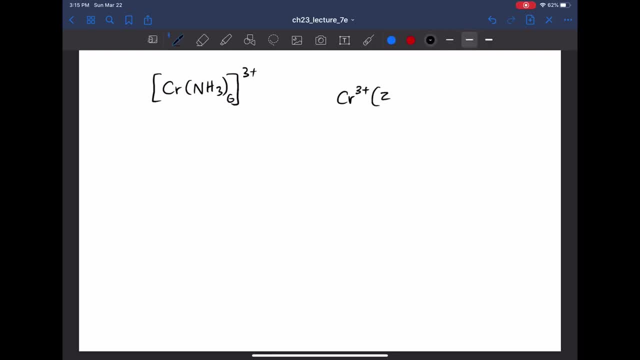 here has an atomic number of z equal to 24.. So when you draw the table, you get 4s, you have 3s, so you have 3s and 3d. So the s orbital has 2 electrons and the d orbital 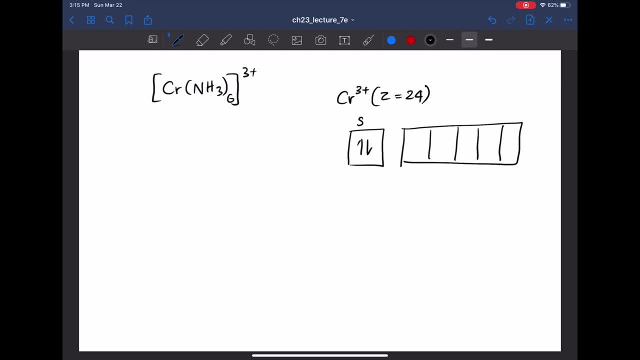 here has, it is 24.. So we have argon 3s2, 3d4.. So it has 4 electrons here. So we have 4 electrons here. But I told you that chromium has a peculiar characteristic where it does. 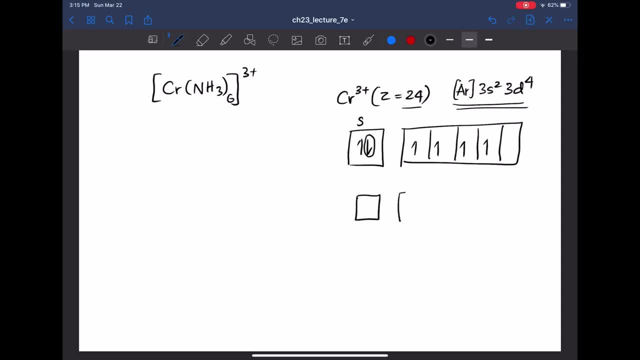 not fill the s orbital, but rather fills the half filled d orbital. So it half fills everything. So this results in all of them having 1 electron each. So now what happens? Chromium, when it becomes Cr3 plus, loses its 3 electrons. So 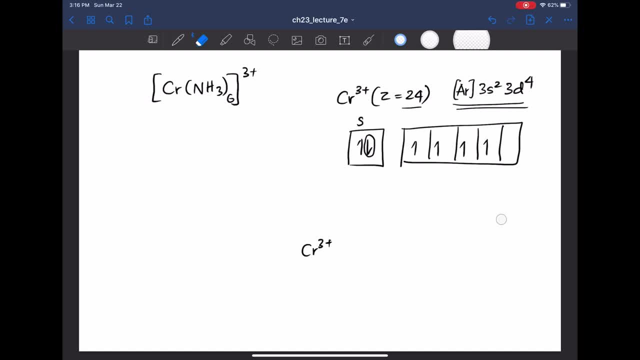 when you consider that, since it was originally just chromium, then we could have half filled orbitals. But chromium here is losing electrons. So I already told you that it losses electrons first in the s orbital. So it loses electrons here first, And then it loses 2 electrons. 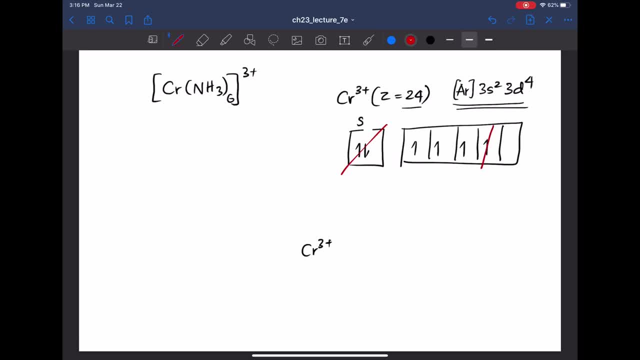 there is lost And then there is another electron here. Now, for just Cr3, you have 3 electrons in the d orbital. Now let us consider that this is a chromium. This is a chromium, This is a chromium here, But we consider that this is a chromium and this is an argon, And 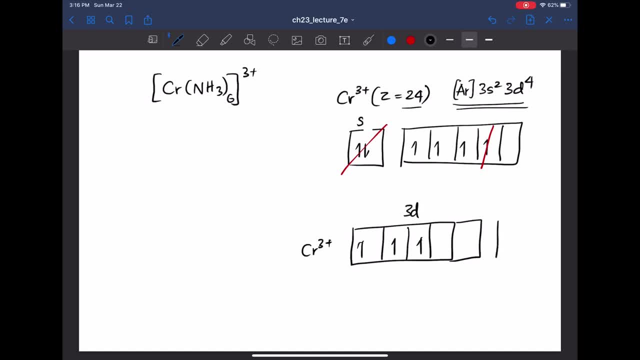 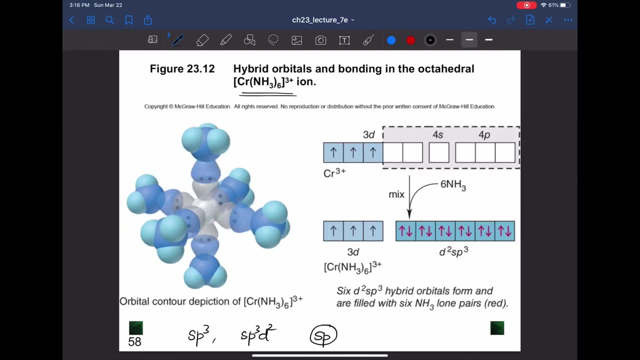 the d-orbitol, and we can consider the next orbital as well. The next orbital here is 4s-orbitol and the 4p-orbitol. So what happens in this hybridization here, in sp3 hybridization here? 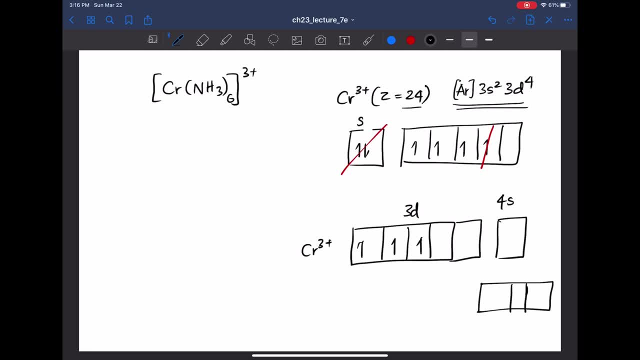 is that it combines the rest of the 3d orbitals, the 4s-orbitol and the 4p-orbitol. So you have two of them here plus one, and from the 4p-orbitol you have another three, The combined here of s. 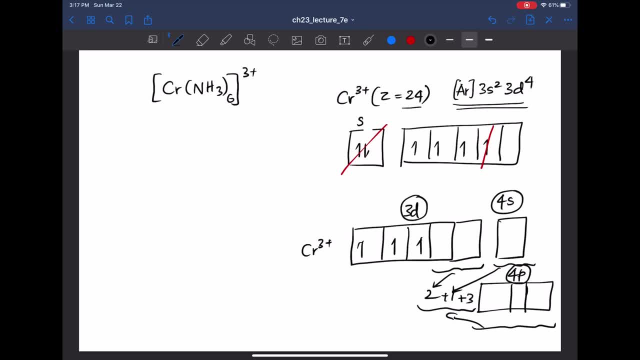 p and d. where s donates two electrons, it becomes sp p3, and then it donates three pairs and d has two pairs, So it forms sp32 hybrid orbitals. So the combined orbitals then form a sp3-orbitol. 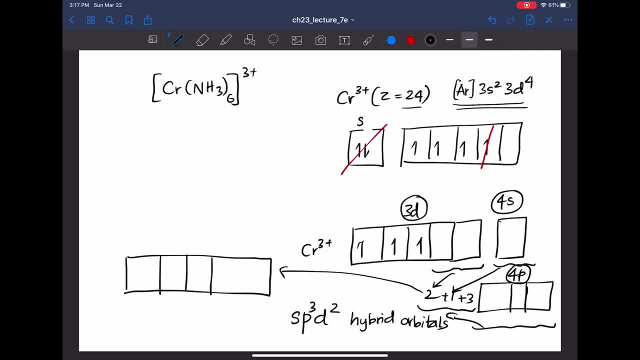 So this is 6 series of orbitals. So this is 6 sp3 d2 hybrid orbitals. Each ammonia has a lone pair of electrons, So those lone pair of electrons go into each of these hybrid orbitals. So that then results in. 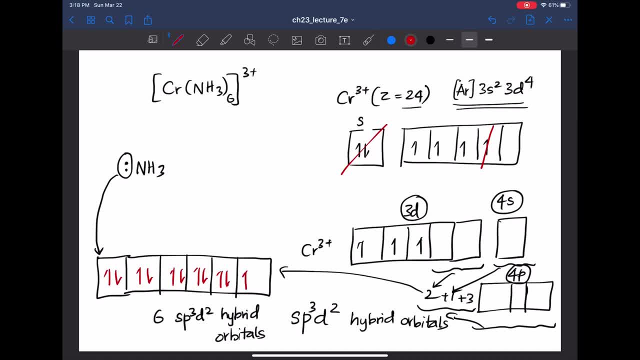 six electron, So six electron pairs from six different ammonia atoms. So you have six of them that are filled in each of these shells. So that's where it forms the coordinate covalent bonds resulting in chromium, hexamine, chromate. So this is how the structure originates. 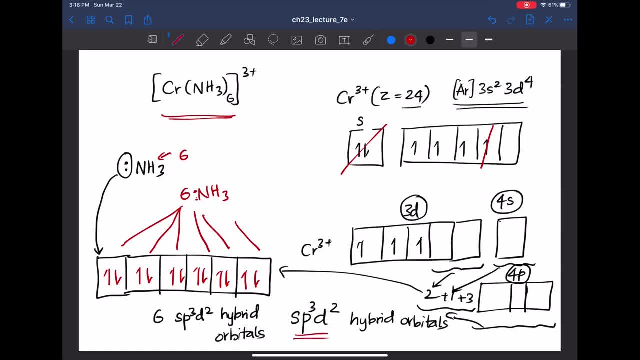 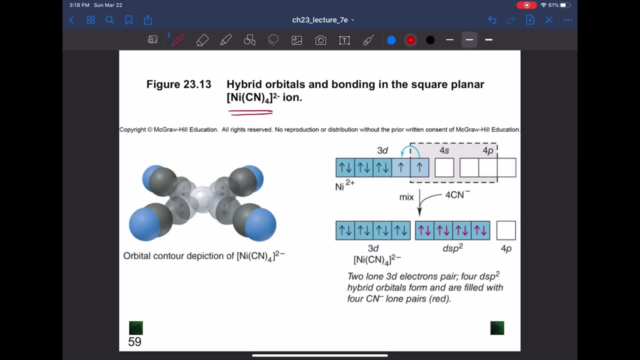 And this is where the hybridization works. Notice that the hybridization here is happening with the empty orbitals that are after 3d. So this is where the structure relies on. When you take the same structure for NiCn4, cyanon, nickel, so you have nickel having Ni2 plus charge, so that results in three lone pairs Nickel. 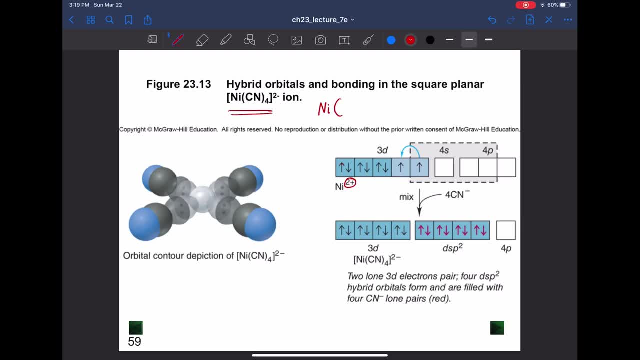 originally has an atomic number of z equal 28.. So you have argon 3s2- 3d8.. So it fills six, three pairs with one electron each, And when it becomes Ni2 plus it loses these two electrons. So what happens now? 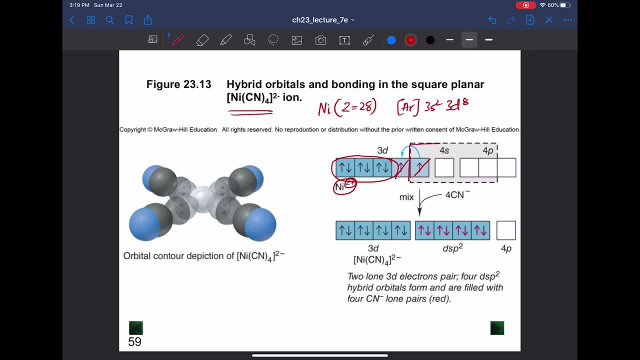 is that it combines the one orbital that it has and it combines everything else. That results in an sp2d hybridization. Those sp 2d you have one s orbital, one d orbital and two p orbitals. So that creates four different sp, two d hybrids. So that, born to four different sp, two d hybrids. 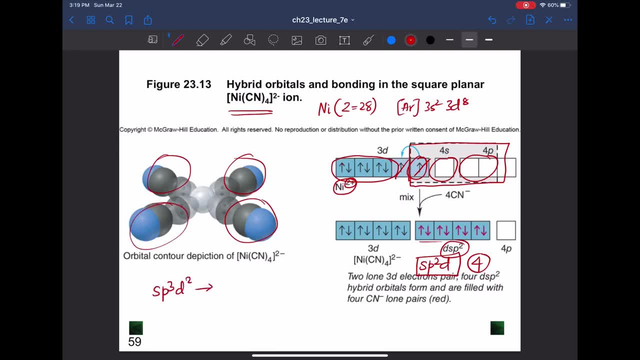 So remember that when it forms an sp three, d, two, the structure is octahedral. For sp 2d, the structure is octahedral, So that's where this covalent bonds get connected in and they get re- castle out of it. So this is where 이b button is and √2 spent on the Io, Nso사�andhize is 통choincluded in each fibre composites. 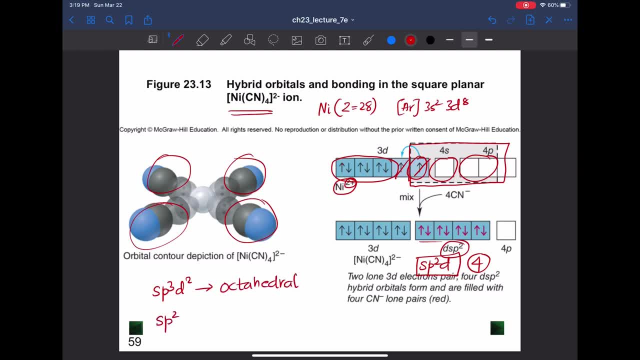 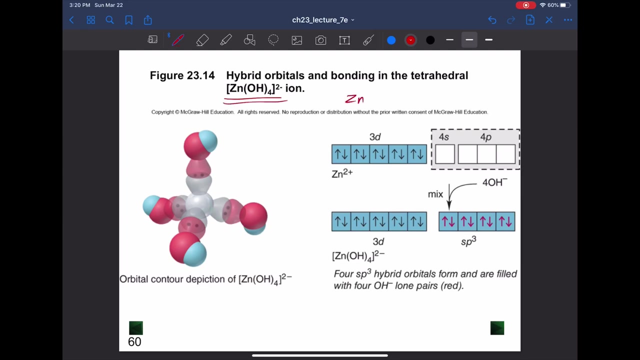 for sp2d, the structure is square planar. so then, when do you get a tetrahedral structure? you get a tetrahedral structure when it forms sp3 hybridization. so that is the next structure, which is for zn, oh taken for, and zinc has no d orbitals left, so the orbitals taken are the next. 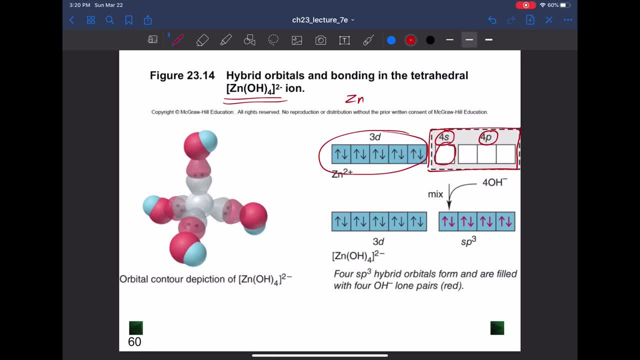 orbitals 4x and 4p. we have one 4s orbital and three p orbitals. it forms sp3 hybridization, so four oh ions donate each electron pair and then form sp3 hybrids. so when it has sp3 the structure forms a tetrahedral structure. so this is the summary of the structure. 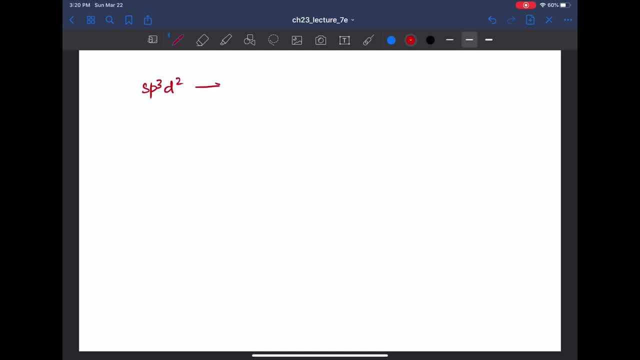 so at what time we get what structure? if it sp3d2, we have six bonds, and so so we have six ligands. that results in an octahedral structure. if you have sp2d structure, you form four bonds with four ligands, and that creates a square planar structure. 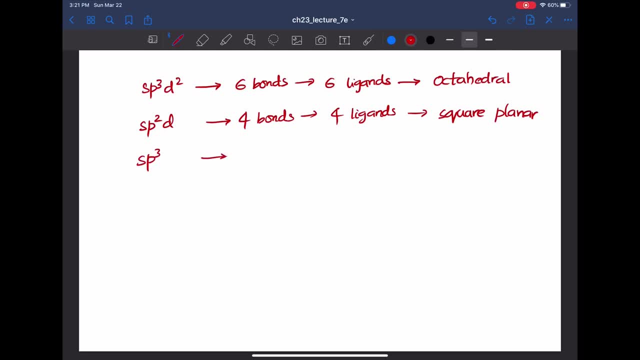 and if you have sp3, you still form four bonds with still four ligands, but you end up with a tetrahedral structure. so here the angle between each of them is 90 degrees in the equatorial direction and 90 degrees in the axial direction. in square planar the angle is 90 degrees. 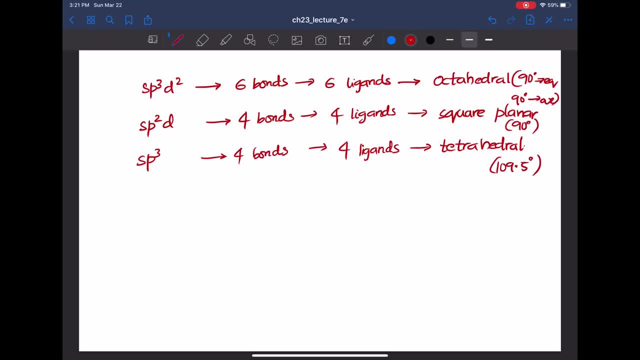 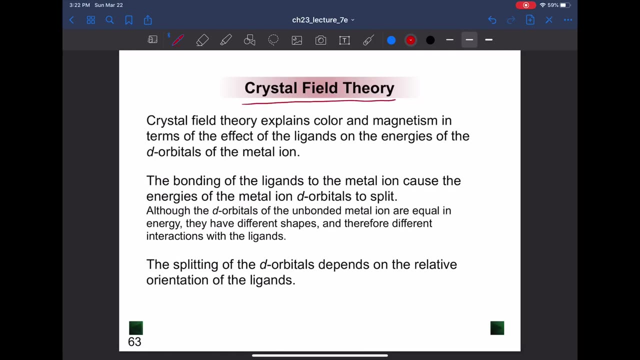 in tetrahedral the angle is 109.5 degrees, so this is the angle and the structure that determines. so the hybridization determines the structure that is obtained. so the next topic is the crystal field theory. so crystal field theory is the crystal field theory, so crystal. 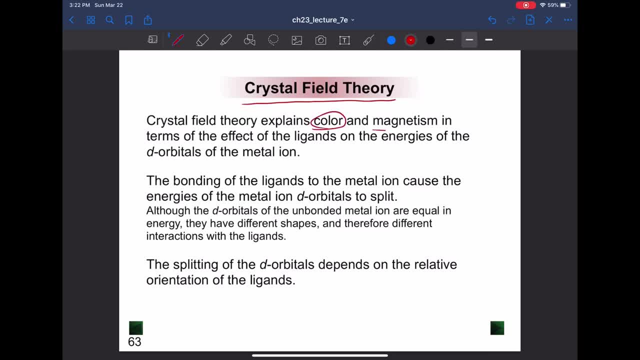 field theory basically explains why transition elements end up with color and magnetism and the effects of ligands in creating the color and magnetism. so the bonding of ligands to the metal ion cause the energies of the metal ion in the d-orbitals to split. so how would the splitting of the d-orbitals occur? so splitting? 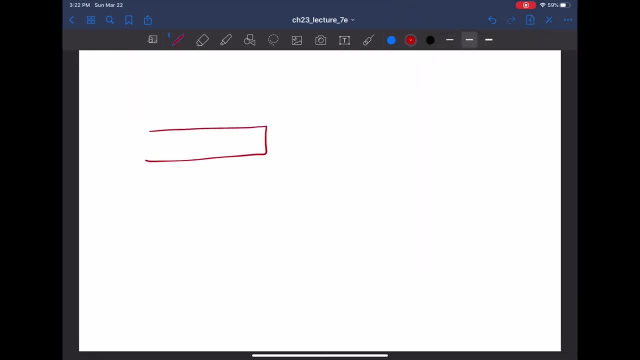 in general you have a 3d orbital with five different pairs. this 3d orbital, when it bonds with ligands, it reaches a higher energy because of the extra electron. then this again splits into two parts: one with a lower energy, one with a higher energy. so two of them go to higher energy and three of them go to lower energy. 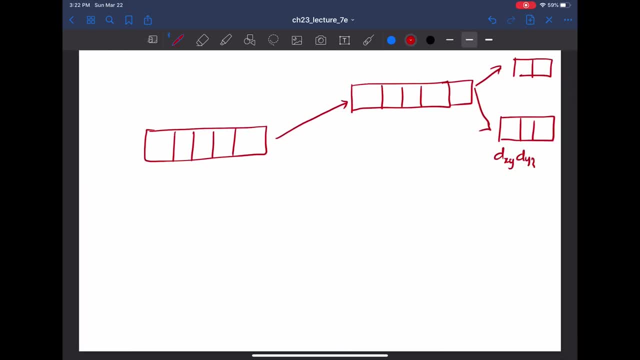 the three of them that go to lower energy are d x, y, d y z and d z x, and the ones that go to higher energy are d x square minus y square and d z square. so this, the energy difference between the last split between these two orbitals, is called delta. this energy is called as: 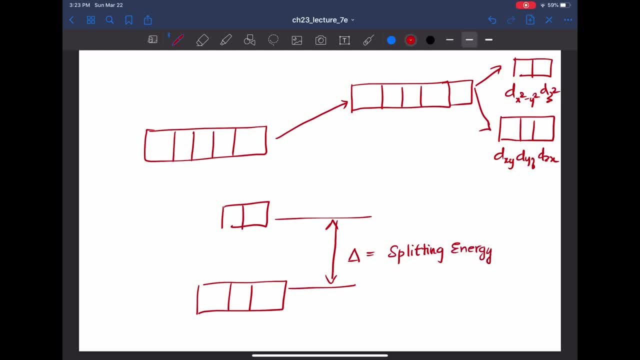 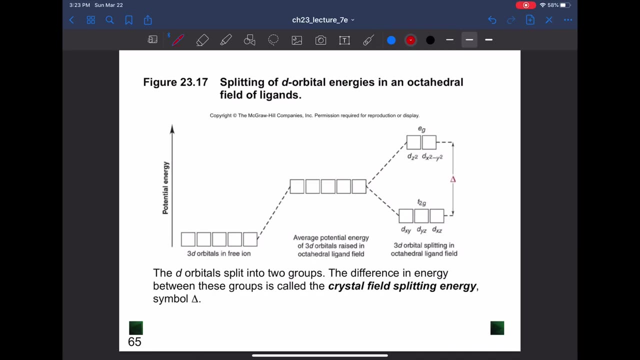 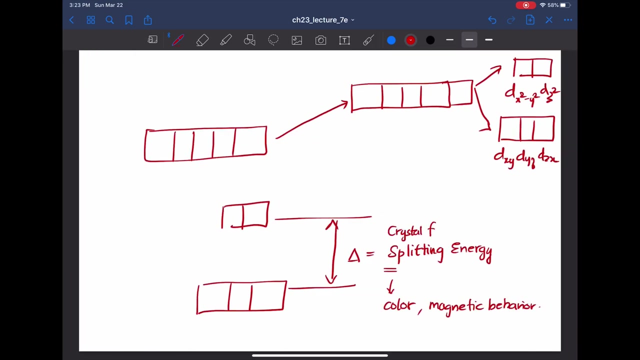 the splitting energy, so this energy is called as the splitting energy, and this is the energy that can determine the color and that can also determine the magnetic behavior. it can also determine the magnetic behavior, so this splitting energy is also called the crystal field splitting energy, so this delta energy is called as the crystal field splitting energy. 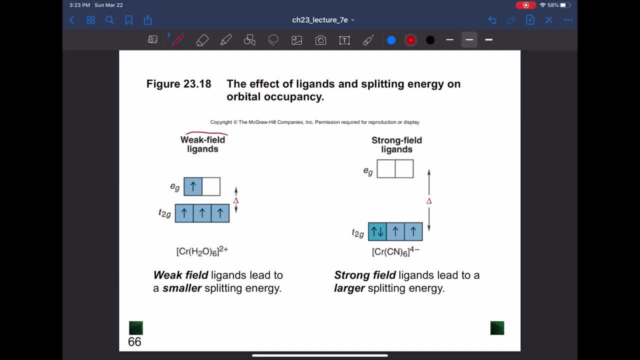 so this will also determine the κά num and which isuman legan. and that is super uh. now, when you have a weak ligand, the ligand or weak field ligands, they are weak field ligands when the splitting energy is small. you have a strong field ligands and the splitting energy is large. 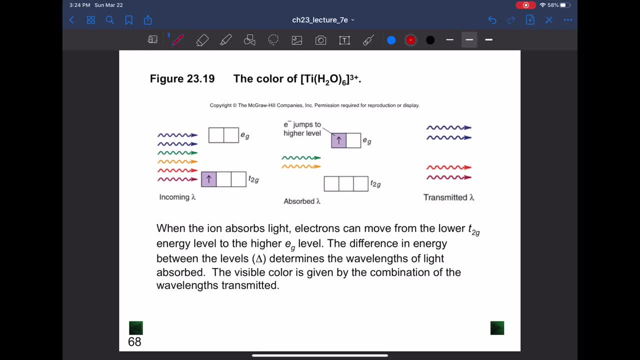 that is determined by the ligands that we use. how do you get the color of titanium here? titanium, hydroxide, titan, so hexahydro, hexa, aqua, titan, titanate has a splitting energy of a really small amount, so the amount of light that passes through this energy determines what light passes through this. so here the gap is only left. 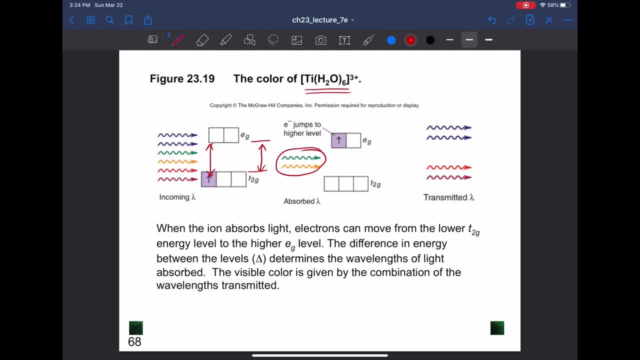 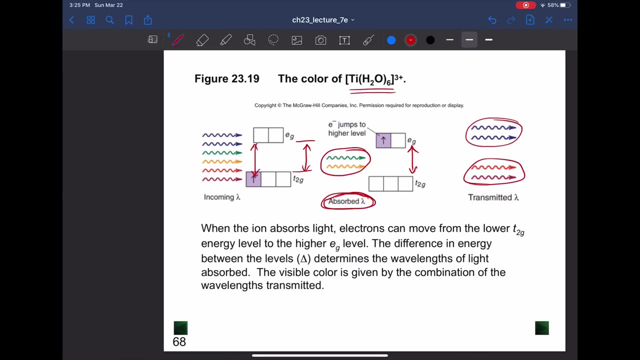 for green and yellow. so then in the second part it's absorbed and then transmitted. so what happens here is that whatever is the energy split, that energy is absorbed. whatever is the rest is left out. so what is absorbed is what the combined color looks like. so here it absorbs green and yellow. so 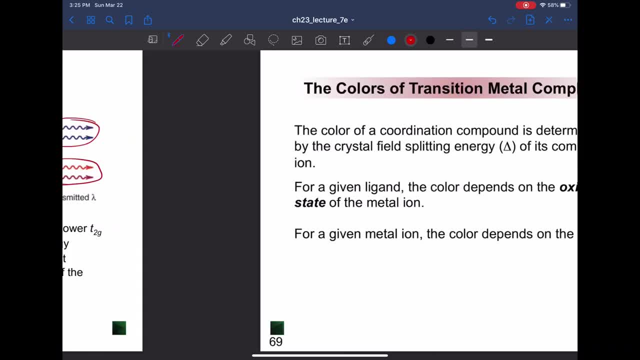 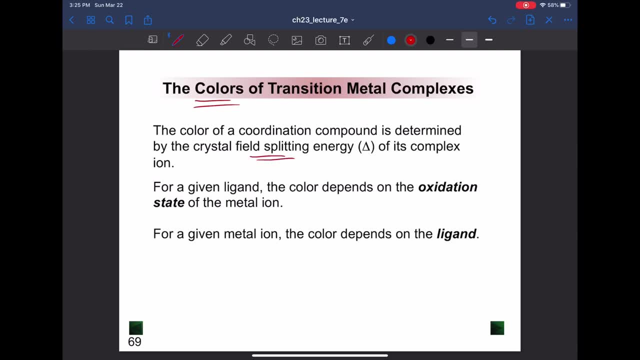 the combined color gives you a purple color. now the colors of the transition metal complexes can be determined by the crystals field splitting energy of the complex ion. so for any given ligand, the color depends on the oxidation state of the metal ion. so the color depends on the ligand. now if you consider vanadium hydroxide, where the oxidation 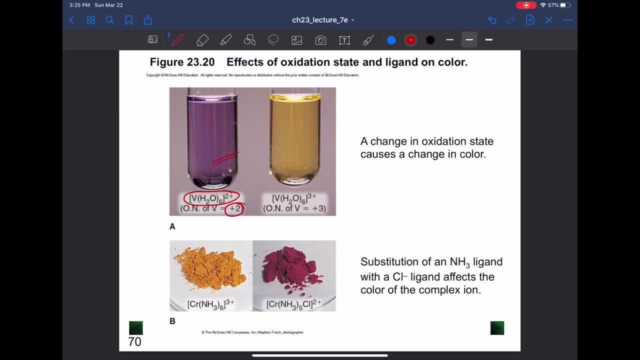 number is two plus two, it has purplish color. when it is plus three, it gets an yellowish color. in the same way if you take chromium, hexamine chromate, so it results in a yellow color. where the chromium has different chromium has three plus oxidation number. if it has a two plus, 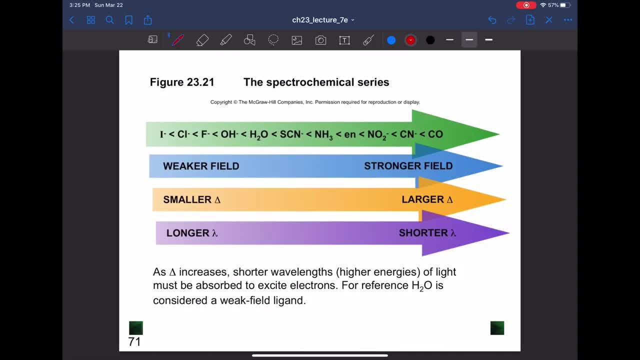 oxidation number, it turns a little more pinkish how to determine the spectrochemical series. so the more the charge on the ligand, the weaker the field. again, the more as you go from, iodine is the one that is the weakest field. again you go to copper monoxide, which is the strongest field again and it results a smaller wavelength. 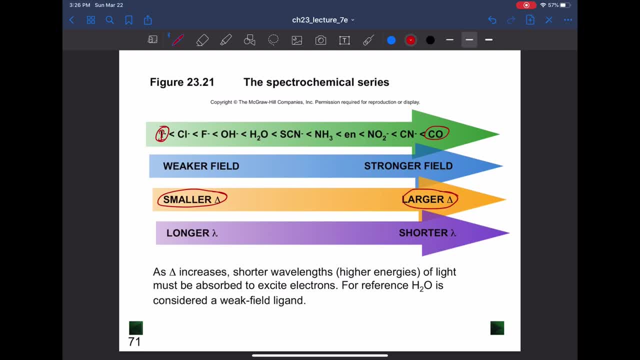 smaller energy to a larger energy, so and you go from a longer wavelength to a short wavelength. so as you increase the delta value you start to get a little bit of a pinkish. so this is the seeing shorter wavelengths of light and must be absorbed to excite the electrons, For example. 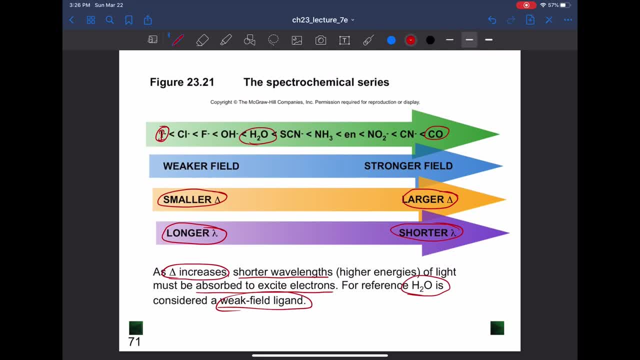 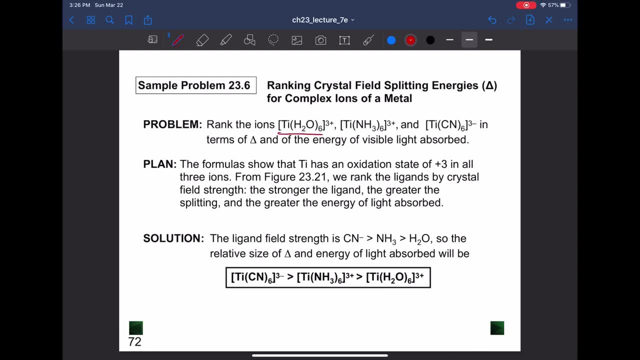 H2O here is considered a weak field ligand and in consideration NO2- is considered as a strong field ligand. So let us compare here between titanium, where you have H2O ligand, NH3 ligand and Cn ligand. Now we are ranking them based on delta and energy of the visible light absorbed. 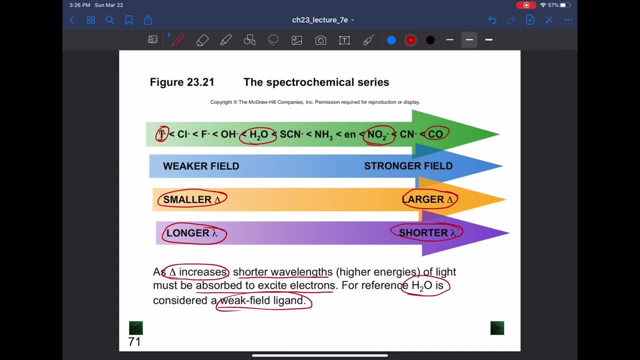 Now let us look at each of them in this diagram. Now we are talking about these three compounds, So we are looking at H2O, NH3 and Cn. So in place of splitting them with in terms of delta, we are looking for the smallest delta value to a largest delta value. 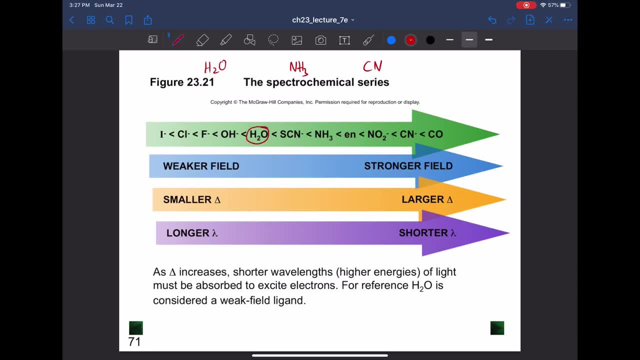 So in the series H2O is first, next you get NH3, next you get Cn, So TiH2O. so here we can write: H2O is less than NH3, less than Cn minus. So this is for delta. In terms of the next part, 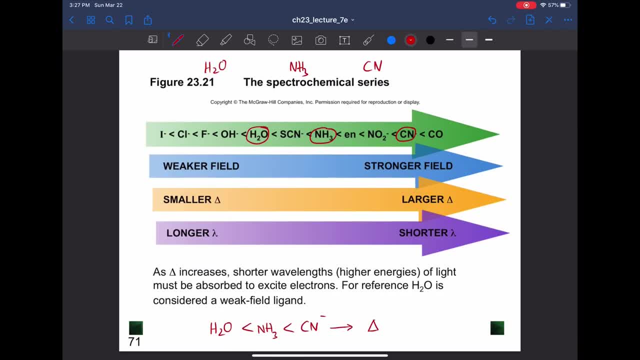 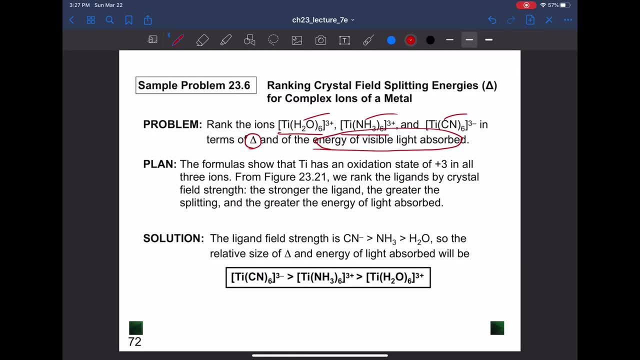 which is the energy of the visible light absorbed. So visible light is absorbed more when you have a lot larger structure. So the same thing happens here as well. So you end up with a smaller, larger delta to a shorter delta, So more energy is. 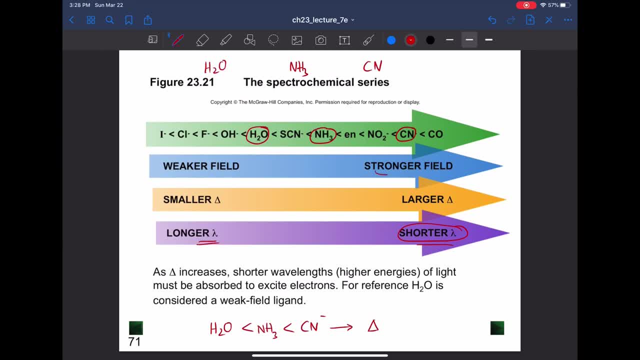 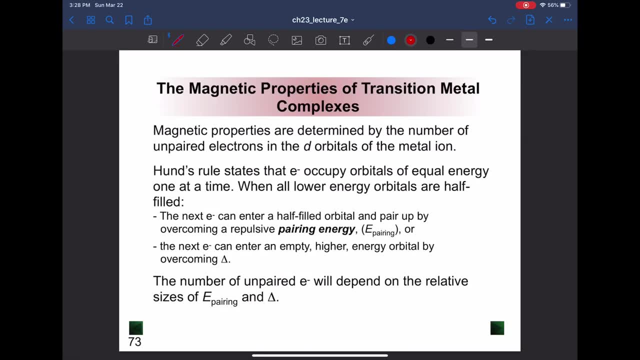 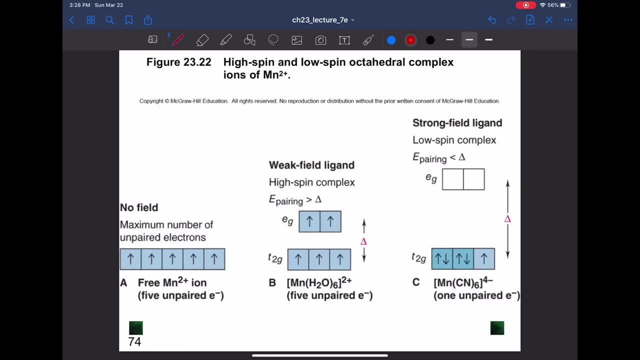 absorbed by the shorter delta region. So because it is a stronger field than a weaker field. So this is your final answer. Now how do you classify the magnetic properties? So magnetic properties are determined by how excited the electrons get. So if you look at a general magnesium manganese atom, Mn2 plus has about five. 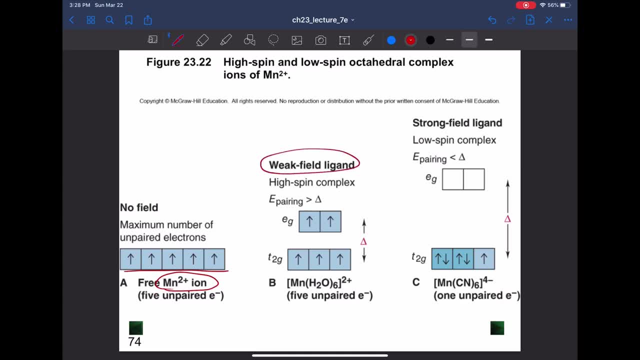 free electrons When it is a weak field ligand that comes in. when you take MnH2O, the splitting energy is smaller, So it has a high spin complex where the electron jumps easily from one orbital to the other. So it is easy for the electrons to jump from a lower energy orbital to a higher. 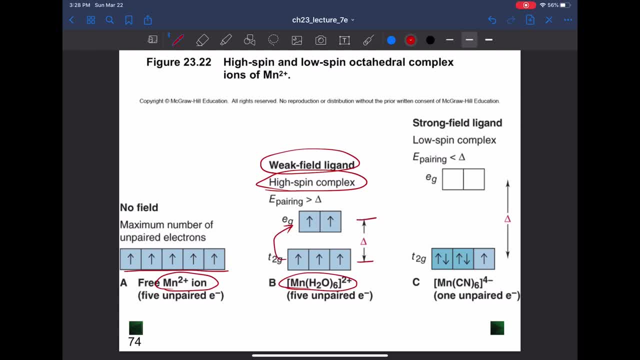 energy orbital, So it goes from here to here. But when you have a strong field ligand, less than say, for example, Cn, it results in the electrons not able to go to the higher orbital, resulting in the electrons going, staying at the lower orbital. So this is the energy called as. 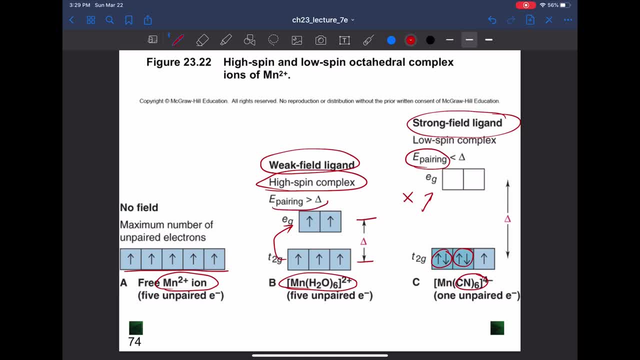 the energy of the pairing. So if the pairing energy is greater than the splitting energy, that results in a higher magnetic field. If the pairing energy is less than the magnetic energy, this would be. if the pairing energy is less than the splitting energy, that results in a 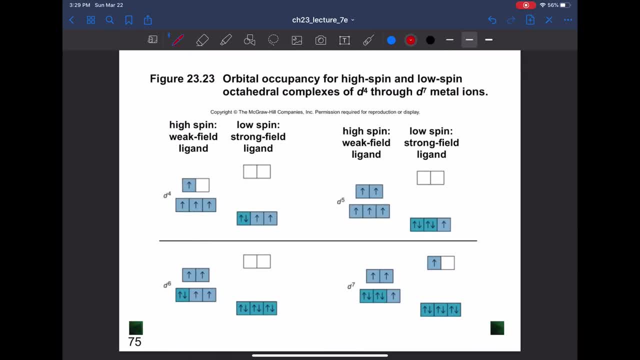 stronger field. So again here you have D4, where high spin results in a weak field ligand where it is easy to jump from one orbital to the other. But here, when you have a low spin strong field ligand, you notice that the electrons cannot jump from a lower orbital to a higher. 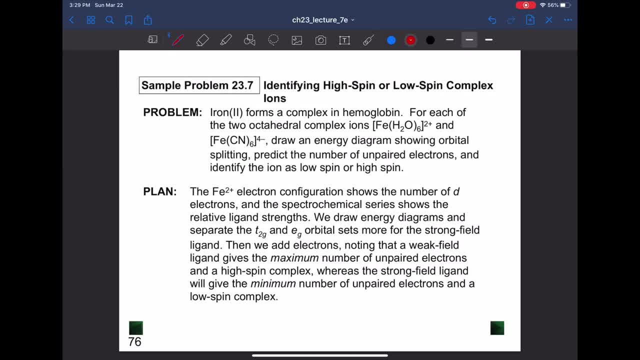 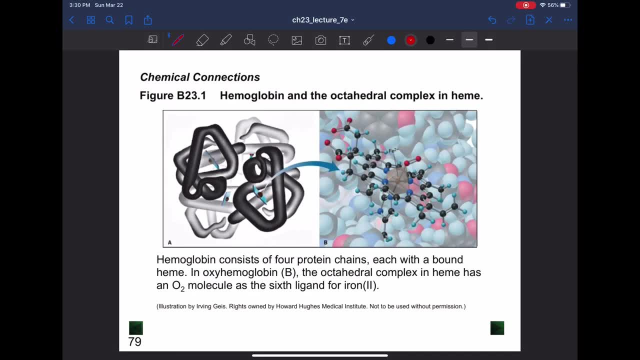 orbital easily. So try this problem and see if you can work out between these two systems. So one last topic to discuss is: why do we need these transition elements? One common connection is the concept of hemoglobin and most common essential enzymes and vitamins. Most common essential enzymes and vitamins generally have a metal. 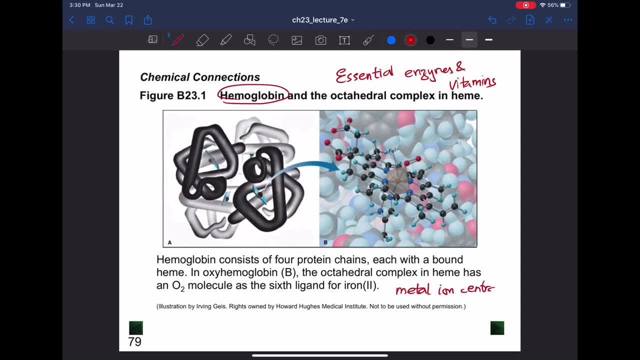 ion in the center and they are generally complex ions, So most of them are complex. So the best example of this is hemoglobin. Hemoglobin has a central compound which is the main active compound, which is heme. Heme contains a small iron molecule in the center. 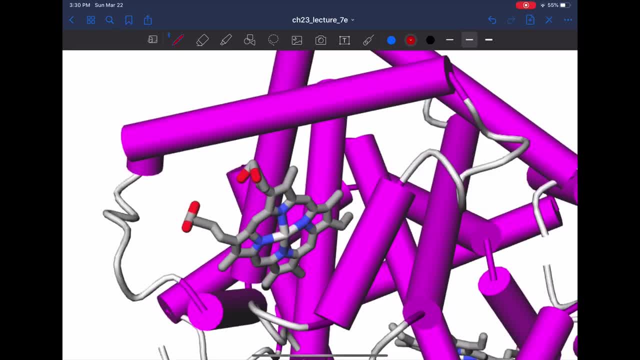 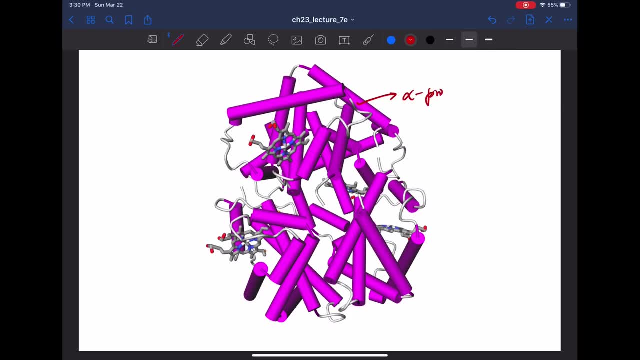 So the best example of this would be this structure. So here, this is the protein heme. So everything that you see here, these are alpha proteins And I want you to focus on this ligandic structure. so this structure. 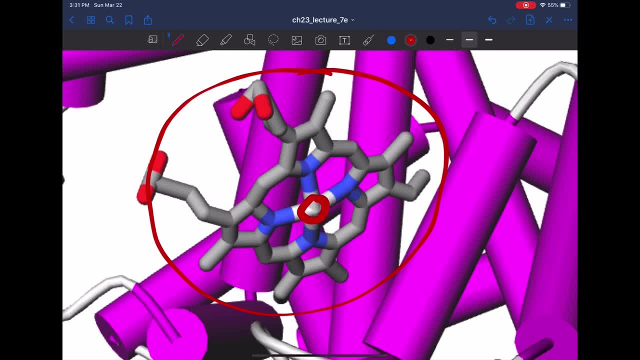 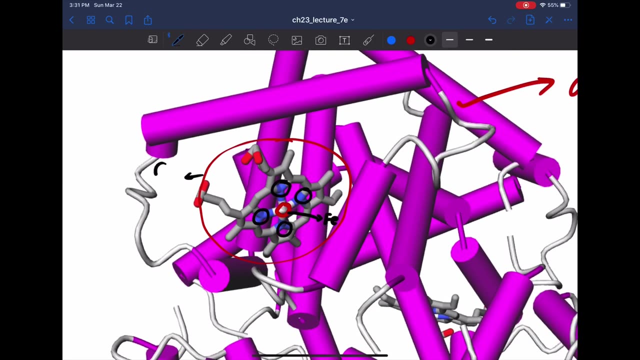 In this structure. this is the iron molecule. So this is the iron molecule. heme And all of the other structures that are connected to them form the molecule. So this is what carries oxygen. So this is what carries oxygen. 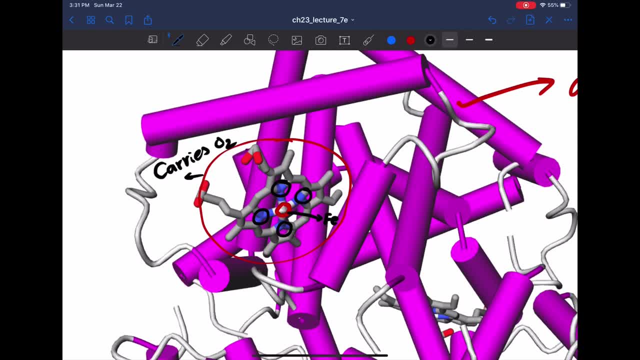 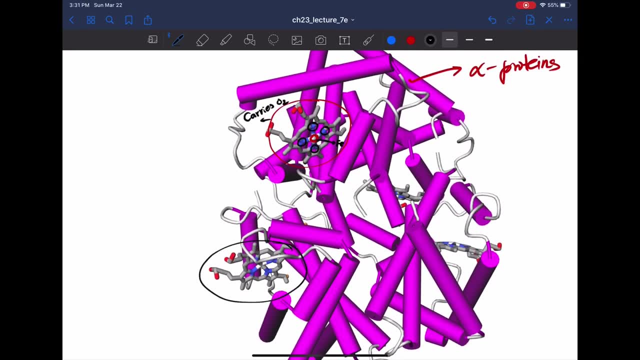 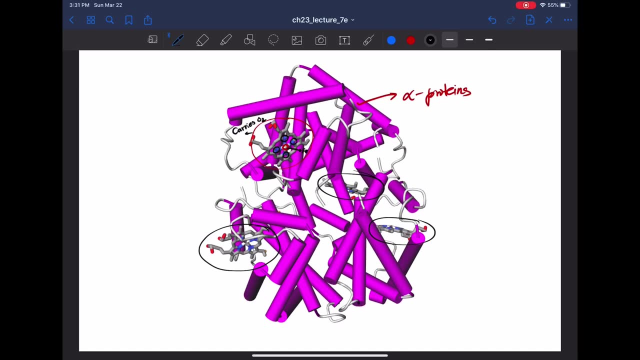 This is the central ligandic molecule that can carry the oxygen. So these are some of the common compounds. Another example of this comes, so you'll see that each hemoglobin has multiple ones of these. So this is the general structure that you will generally see for any general compound. 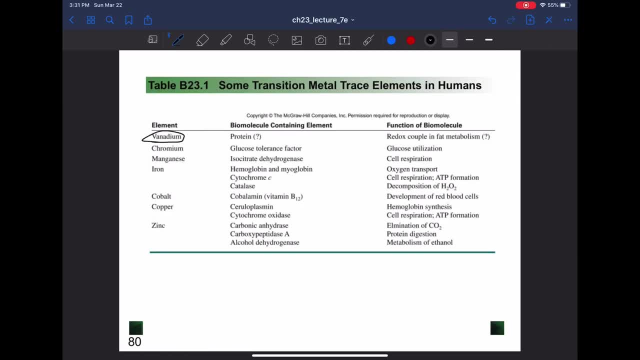 There are multiple of these. Best example of them are: vanadium in proteins that are used in redox couple as a redox couple in fat metabolism. Chromium is used as a glucose tolerance factor and it's used to utilize a lot of glucose. 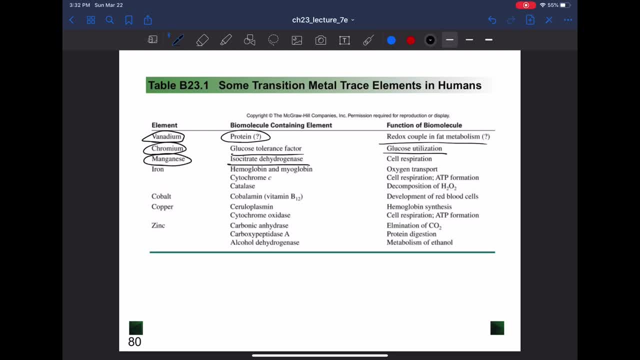 Manganese is used in an enzyme called isomerase. It's a citrate dehydrogenase. It's used in cell respiration. Iron is common in hemoglobin and myoglobin, cytochrome C and catalase In hemoglobin. it's used for oxygen transport. 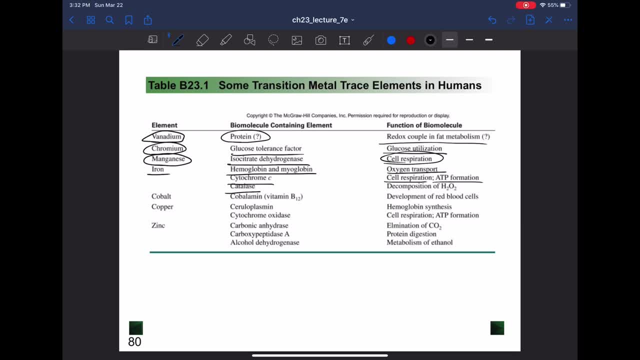 In cytochrome C, it's used for cell respiration and ATP formation. In catalase, it's used for decomposition of hydrogen peroxide, And cobalt is the compound that's found in cobalamin. Cobalamin is vitamin B12.. 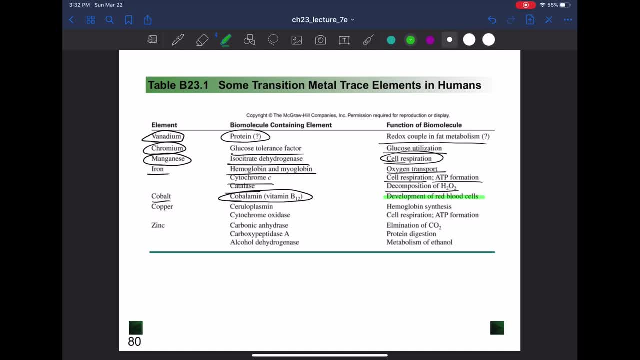 So that's the one that is found there And it's used in the development of red blood cells. Copper is used in two different enzymes: One is citrate dehydrogenase, The other one is cyriloplasmin and cytochrome oxidase. 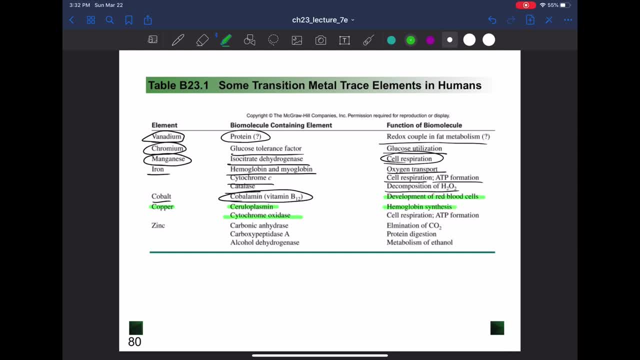 Cyriloplasmin is used in producing hemoglobin. Cytochrome oxidase is used to produce in cell respiration and ATP formation. Zinc has multiple uses. It's also used in an enzyme called carbonic anhydrase, which is used in the elimination of carbon dioxide. 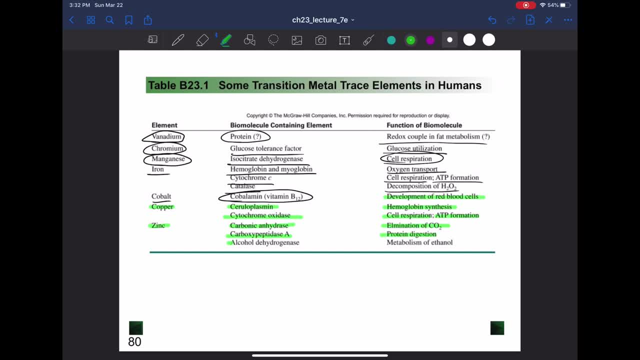 Carboxypeptase A, which is used in protein digestion, And alcohol dehydrogenase, which is used in metabolism of ethanol. So it helps us in understanding how these metal trace, the traces that are present in our body, can help understand the common essential elements that we generally use.